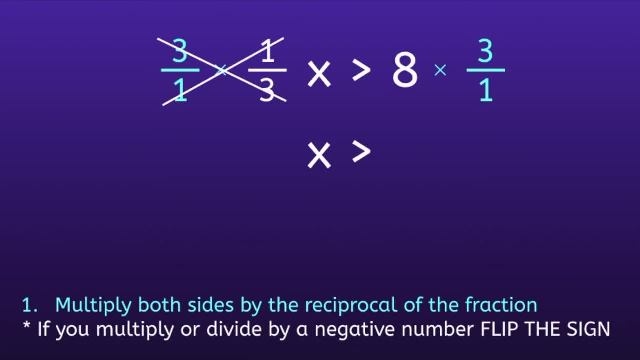 that rule and we can bring down the inequality sign. If I look on the right side, I have 8 times 3 over 1.. It's important for us to notice that 3 over 1 is equal to 3.. So now, 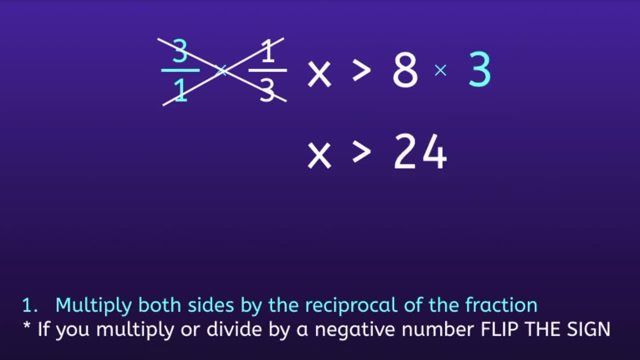 we have 8 times 3, and 8 times 3 is 24.. So the final inequality will be: x is greater than 24.. Example number 2. Negative 1. fourth: x is less than or equal to 3.. Step 1.: Multiply both. 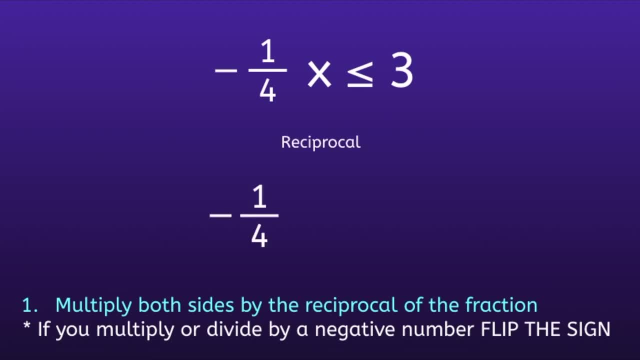 sides by the reciprocal of the fraction. So what is the reciprocal of negative 1? fourth, If you were thinking negative 4 over 1, you are correct. So notice, I keep that negative sign and just switch the numerator and denominator. 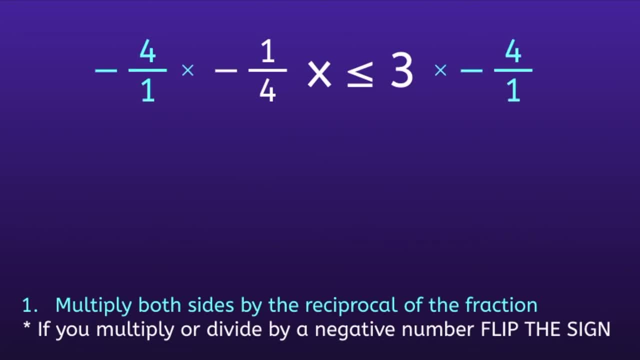 So I'm going to multiply by the reciprocal of the fraction. I'm going to multiply both sides by negative 4 over 1.. If I focus on the left, I have negative 4 over 1 times negative 1 over 4.. I'll pull those out, multiply, which leaves me with 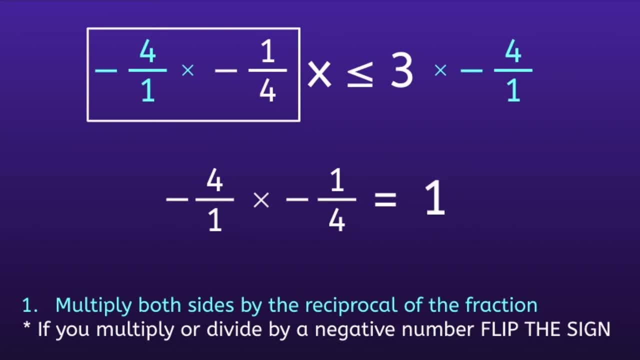 4 over 4,, which is equal to 1.. So, once again, any time you multiply reciprocals, you will always get the number 1.. So we can cross out those 4s, cross out those 1s, which leaves. 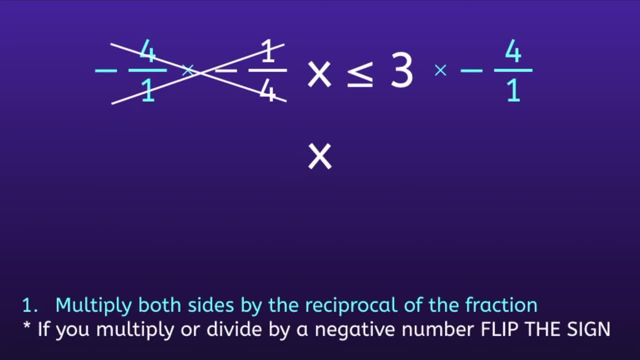 us with 1x. But now it's important to look at the rule at the bottom of the screen. If you multiply or divide by a negative number, flip the sign. Since we multiplied both sides by negative 4 over 1, we do have to flip the sign. So since the original inequality sign 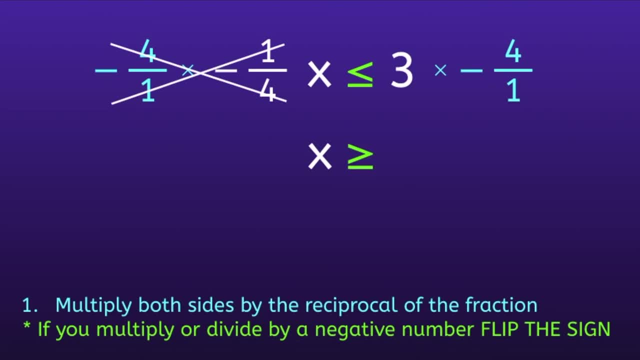 is pointed to the left, we have to flip it. so now it is pointed to the right. If we focus on the right side now, we have 3 times negative, 4 over 1.. And it's important for us to notice that negative 4 over 1 is the same as just negative. 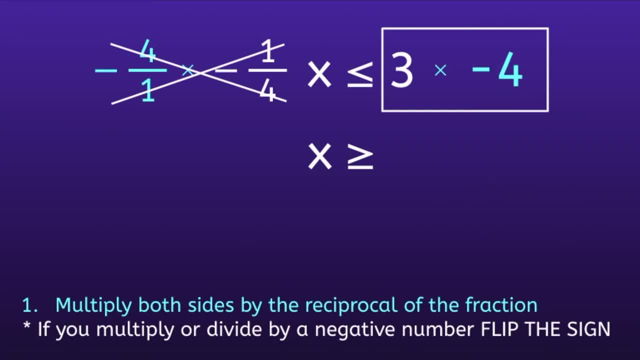 4. So 3 times negative 4 is equal to negative 12.. If you notice you're struggling with multiplying by negative numbers, I will include a link in the description to a song I made to help you with that skill. So the final inequality: